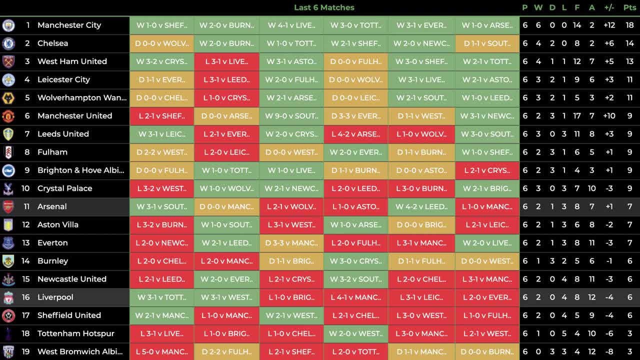 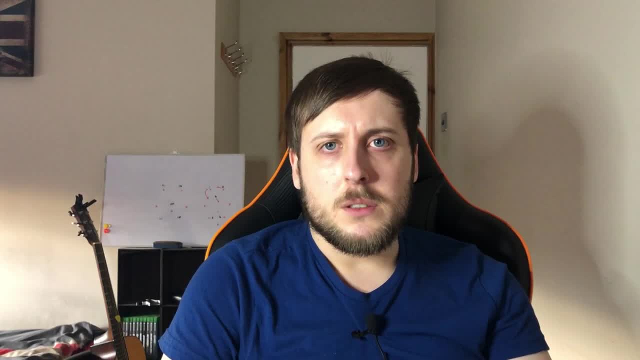 Also, with your pre-game information, you can have a look at form head-to-heads of the teams, just to get a little bit of an idea of how you might expect the game to look. and also, here's my first tip: Just do a quick read of the team that you're going to analyse. 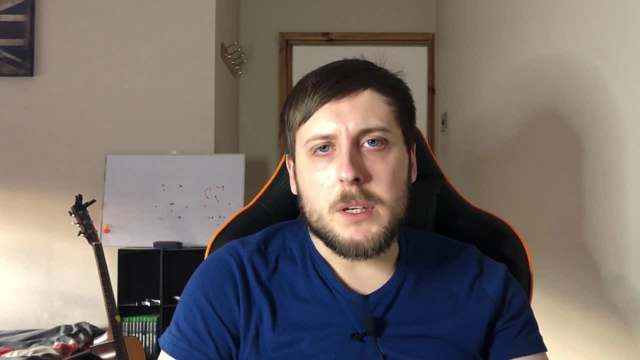 For example, if you're analysing Arsenal, just have a quick read about Mikel Arteta's tactics. This will just give you a little bit of an idea of what to look for while the game's going on, so you're not completely new to it. It's the same for any team- Bielsa's Leeds, for example. just read. 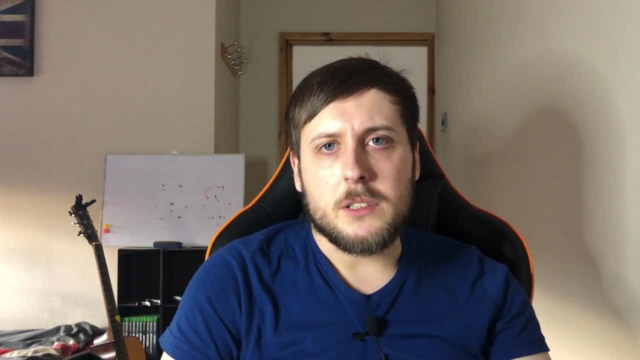 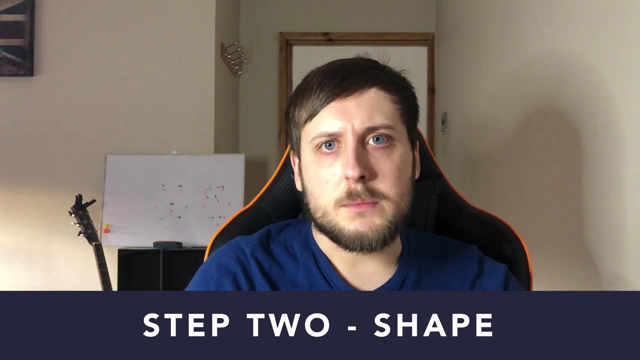 about them. just get that little bit of information in your head so you know what the game's going to sort of look like. So the game's kicked off, and this brings us to step two shape. It's the first thing that would advise you to look for and potentially spend the first. 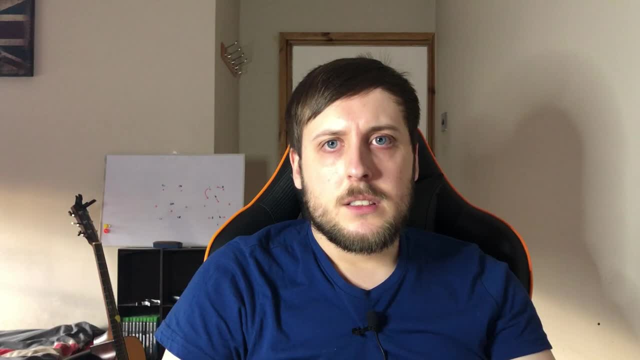 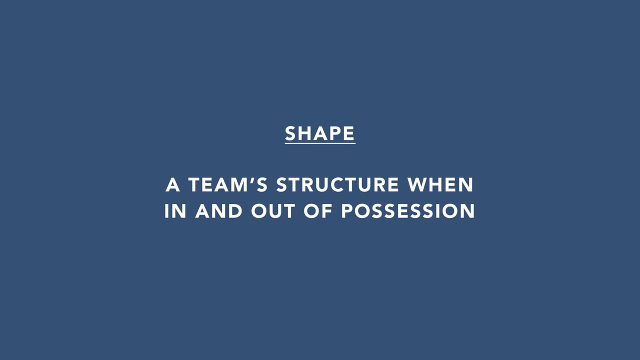 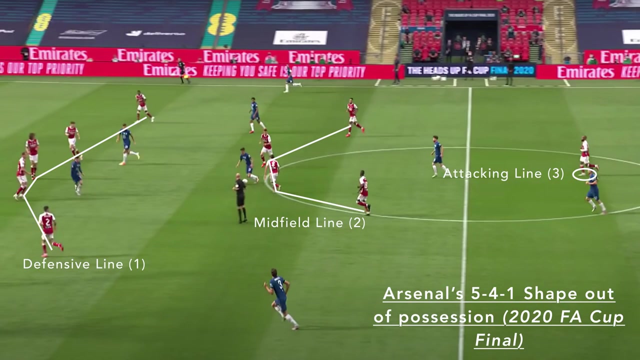 five to ten minutes of the game looking at it. So what do we mean by shape? Well, the shape of a team is how their structure looks in and out of possession. So a team's shape will usually consist of three lines. You can call them defence, midfield and attack, but it will usually be three. 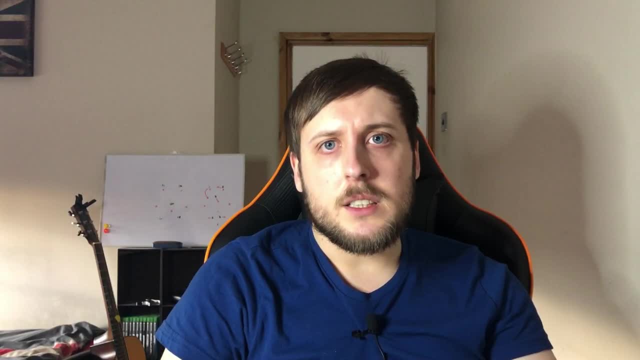 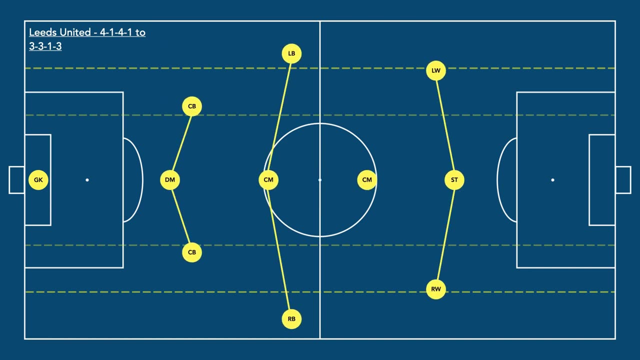 lines. In some cases it will be four, For example Bielsa's Leeds. their shape in possession is a 3-3-1-3.. Most of the time it will be three lines, but there are occasions where it's four. So just try and. 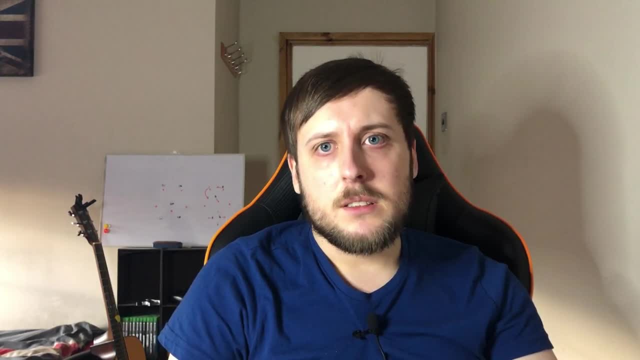 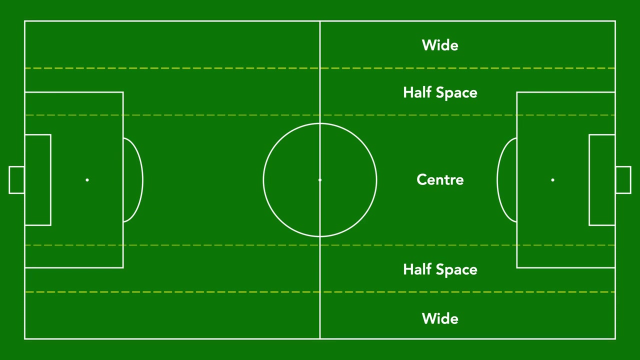 recognise those three lines: Defensive line, midfield line, attacking line. Now, the key here is: just because it's your defensive line, you may not have all defenders in there. There are occasions where a midfielder player might drop in. So if you're not aware of the five vertical zones, try and just make a note of where players are. 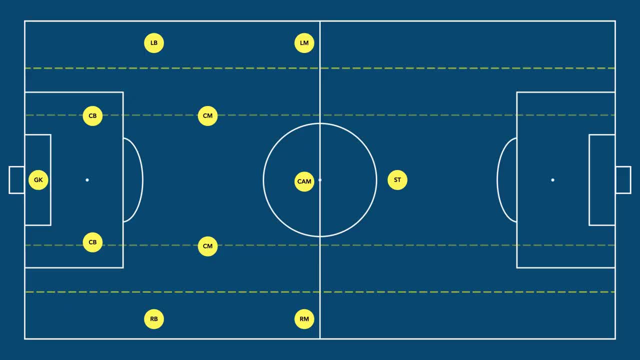 in their shape. So let's take a look at an example. So in our example, the team begins in a 4-2-3-1 formation, but when in possession we notice that their shape becomes a 2-3-5.. So we have our two. 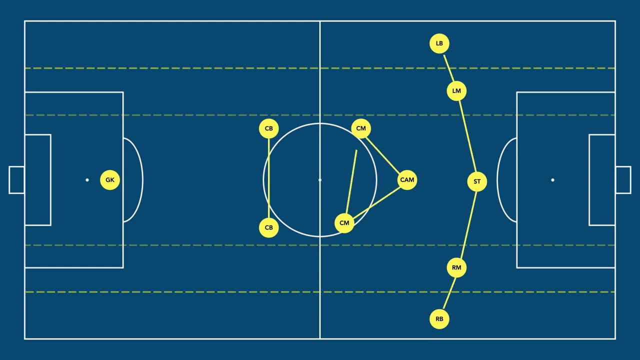 defenders in the first line, our two centre backs. We have our three midfielders in the second line. Now, here's the important thing: to recognise The two centre backs in this shape. they have now joined the attacking line, which consists of the five players, So both full backs, both wingers and the striker, And that's what we mean when we talk. 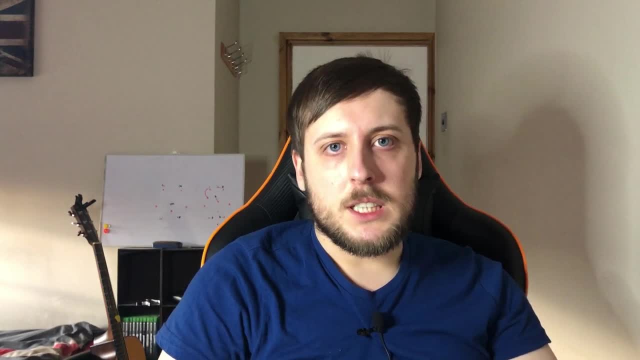 about shape. There will be similarities across teams, but a lot of teams will have different shapes. Just try and recognise the three lines. This is very, very important when it comes to analysis. Don't over complicate it. It becomes very, very easy to make things much harder than they need to do. 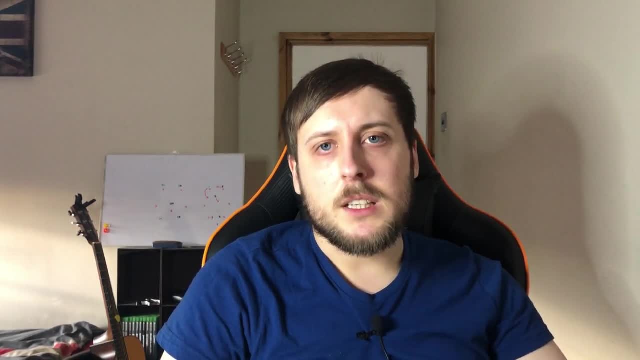 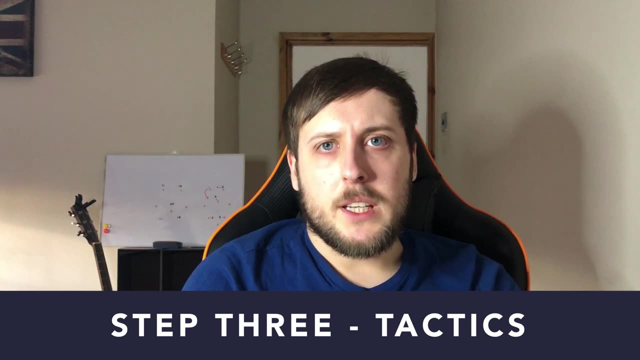 When thinking about a team's shape, just try and recognise those three or potentially four lines. So now we've got the team's shape together, we now get down to the really nitty-gritty analysis. We now need to start thinking about the tactics of the team, both in and out of possession. 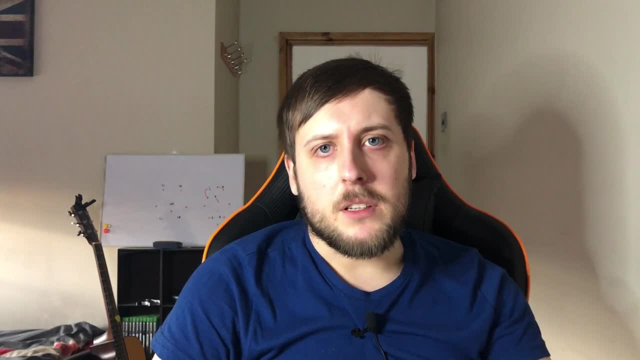 So when the team's in possession, do they play out from the back, Do they play short passes from the goalkeeper and built through the pitch, Or do they play direct? When out of possession, are our team pressing or are they into a deep block? We're now starting to build that really clear picture of what the team's 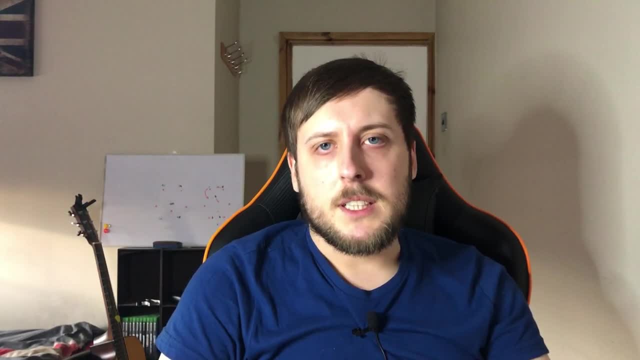 trying to do So. when we're thinking about tactics, this is where it starts to get really different for each team. There again will be some similarities with tactics, but each team tends to have their own sort of set idea of how they want to play. We'll focus on playing out from the back just because 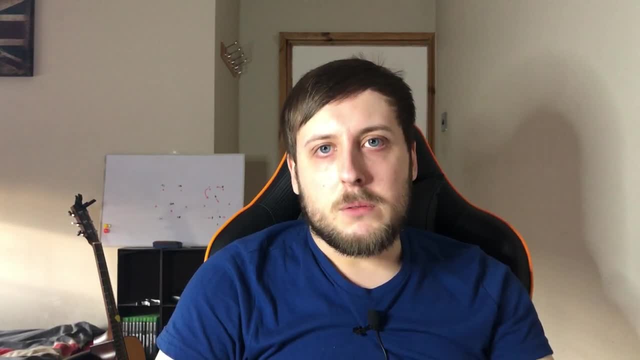 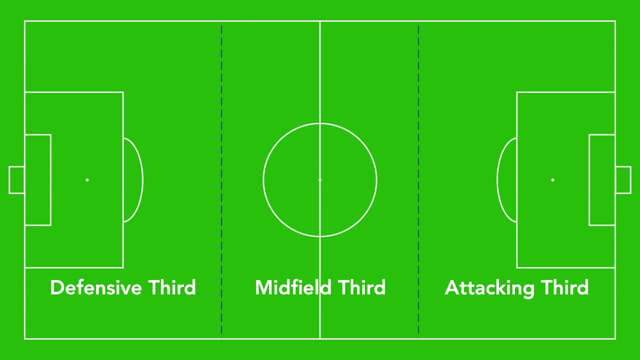 it's easy and everyone knows where it is, But a really good way to recognise tactics is to break the pitch into three thirds. Once you've broken the pitch into the thirds, try and isolate what's happening in each third. So when playing out from the back, first thing you need to think about is the goalkeeper's got the. 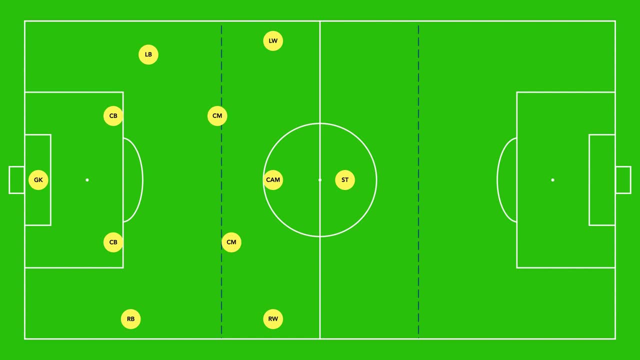 ball. what's the positioning of players like him around? So usually when the goalkeeper's got the ball and playing out from the back, the full backs move high. A central midfielder might drop in to create that initial diamond. So that's your first step. Then it moves into the midfield. 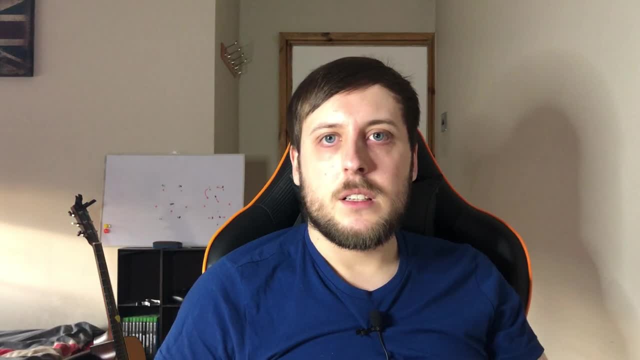 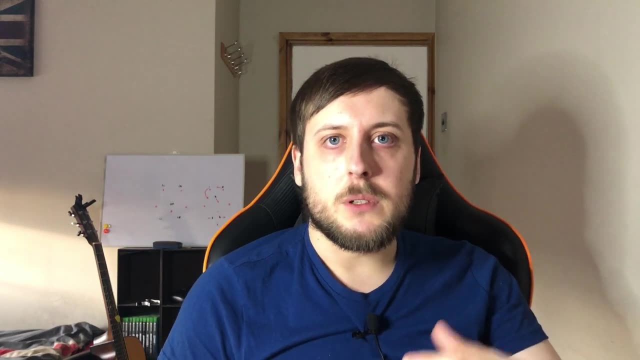 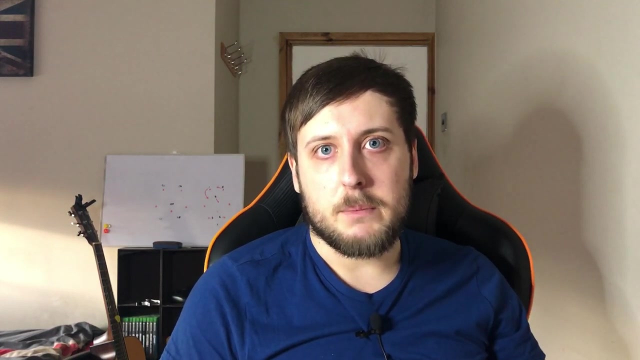 So what's happening in this section? Do the full backs still stay high? Does one invert? What will happen now is, as you progress forward up the pitch, you'll now start to see how the team build into the shape that you put together in the second step And then finally attack in third. 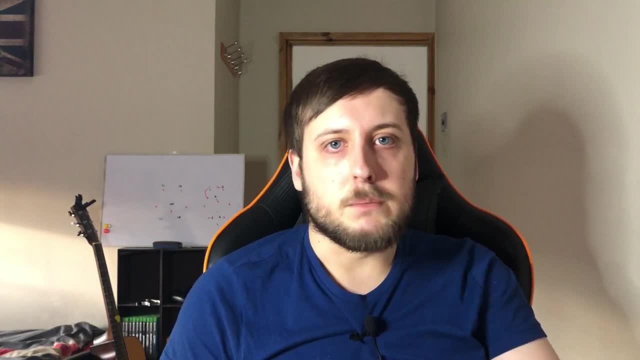 Do they always put crosses in from the left side, Right side? Do they try and break into the box? When we think about tactics, we're now really trying to observe how the team behave and interact with the ball, the opposition and the ball. 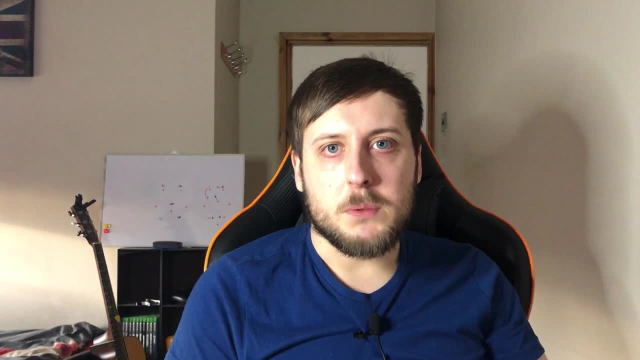 We're now really trying to observe how the team behave and interact with the ball, the opposition, the teammates, players within the same unit, players within different units, And we're trying to recognise whether there are trends. So we'll go back to the goalkeeper Does. 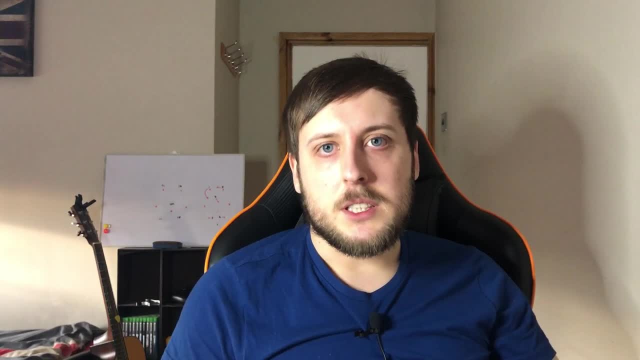 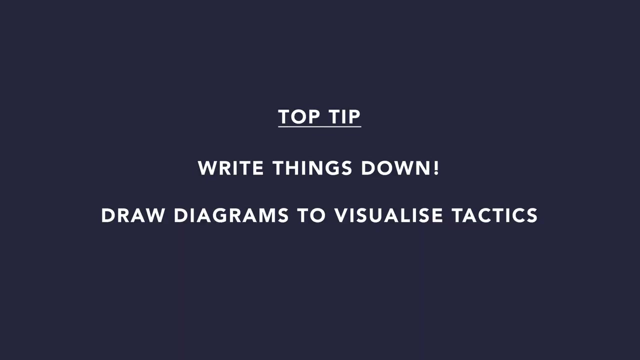 he always play to the left centre back? Does the left centre back always play into a certain midfield player? When that midfield player receives the ball, what happens next? Really focus on details, And a huge tip for this section is: write things down, Draw pictures, draw little diagrams. 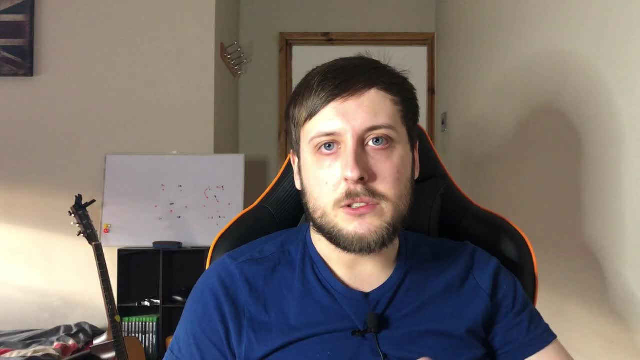 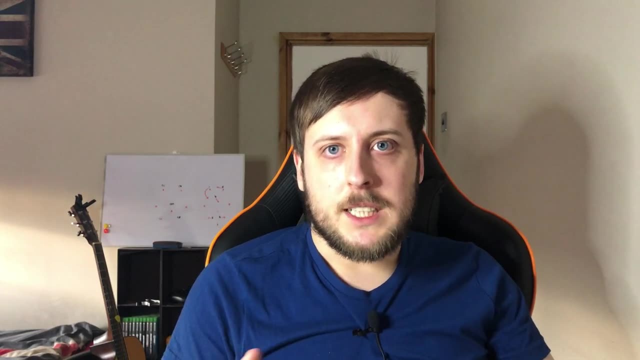 When I analyse football matches, I sit with a whiteboard and I just draw things on it, So it helps me just visualise what's going on. Then, once you think you've got the tactics together and the patterns, really go into detail. So why does this happen when the central midfielder 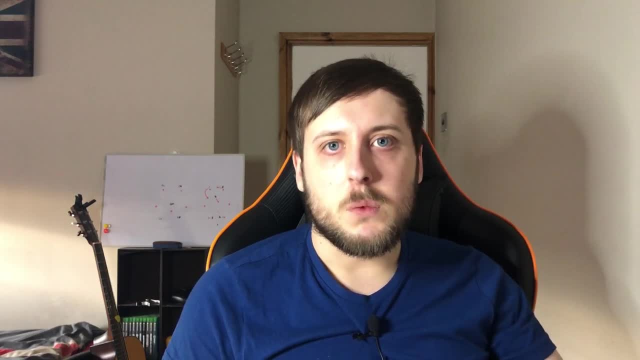 receives the ball. Why does this happen when the striker receives the ball? Why are they positioning like this? What's influencing that? Is it the opposition or is it the teammates that are influencing this? Really, really dig for detail. Just keep asking yourself: why is this happening? 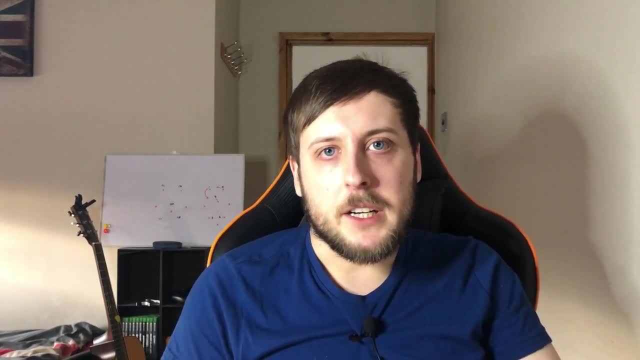 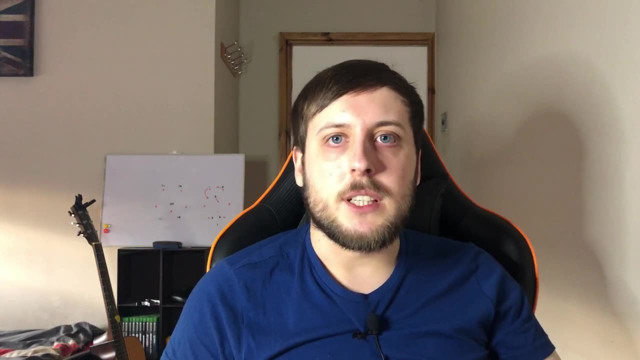 Why does the left back invert? What does that provide? Just keep digging for detail. I appreciate this section is a little bit vague because we're not specifically analysing a team. I'm just trying to give you a few ideas of what you can look for. But this is really. 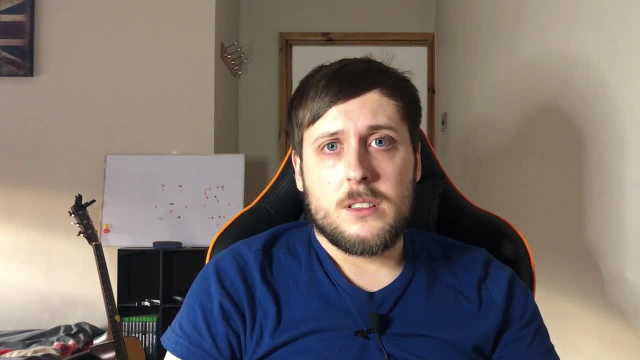 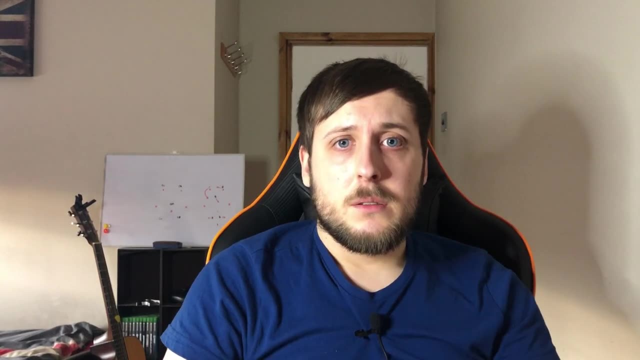 where your analysis starts to take the next step. So that's all the three steps of analysis. So pre-game shape tactics. It takes a little bit of practice to get good at it, But here's a few top tips that can help you along the way.